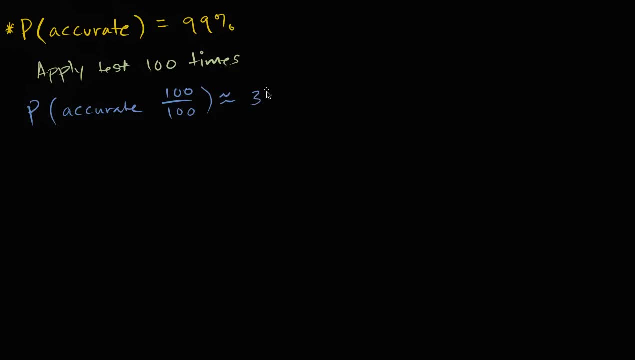 is approximately equal, approximately equal to 36.6%. I rounded to the nearest tenth of a percent, So it's a little better than a third chance that you'll actually get. all of all of the people are going to get an accurate result. 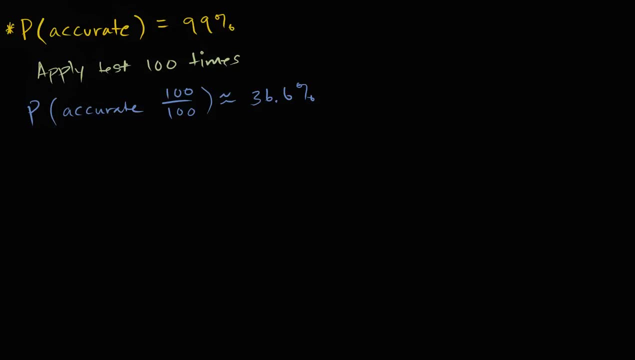 even though for any one of them there's a 99% chance that it's accurate. And we can keep going The probability that it is accurate. I'm just going to put these quotes here so I don't have to rewrite accurate over and over again. 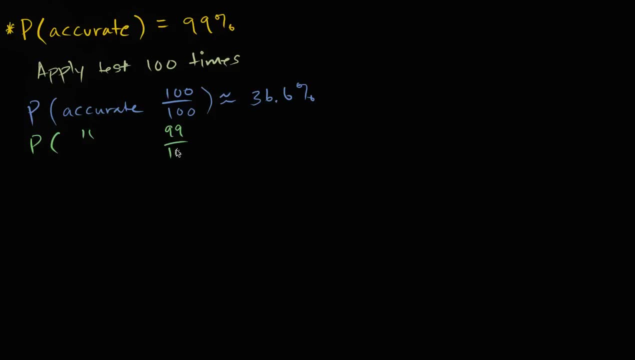 The probability that it is accurate 99 out of 100 times. I calculated it ahead of time- it is approximately 37.0%. So this is what you would expect. Getting 100 out of 100 doesn't seem that unlikely if each of the times you apply it. 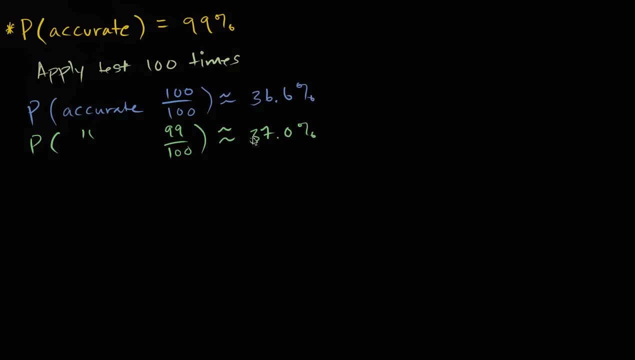 has a 99% chance of being accurate, But it makes sense that you, that you would expect 99 out of 100 to be even more likely, slightly more likely, And we can, of course, keep going The probability that it is accurate 98 out of 100 times. 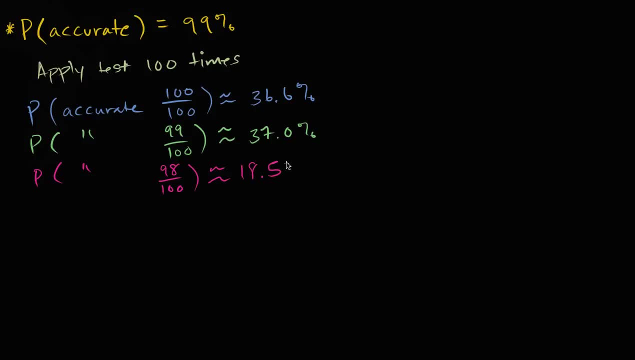 is approximately 18.5%, And I'm just going to do a few more. The probability that it is accurate 97 out of 100 times- and once again, I calculated all of these ahead of time- is 6%, So it's definitely in the realm of possibility. 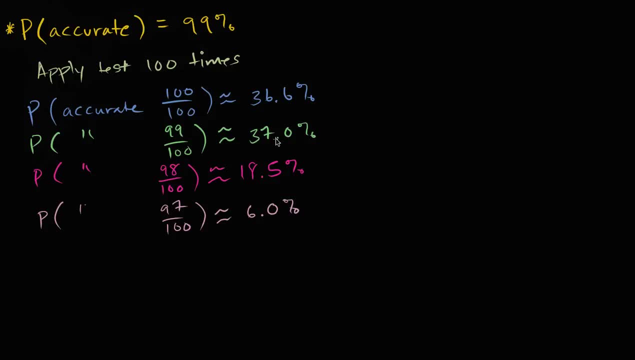 but it's. the probability is much lower than getting having 99 out of 100 or 100 out of 100 being accurate. And then the probability. let me put the double quotes here: the probability that it is accurate: 96 out of 100 times. 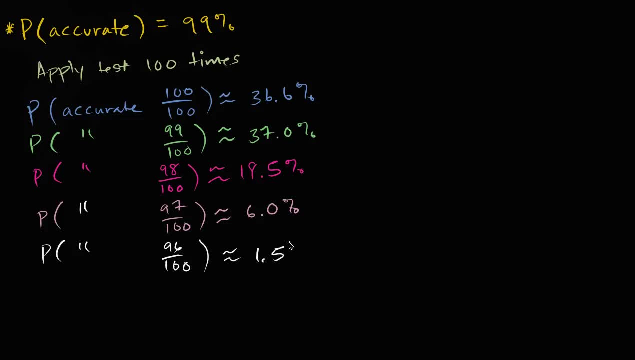 is approximately 100.. So it's 1.5%. And then the probability, and I'll just do one more and I could keep going. the probability: you know, there's some probability that even though each test has a 99% chance, 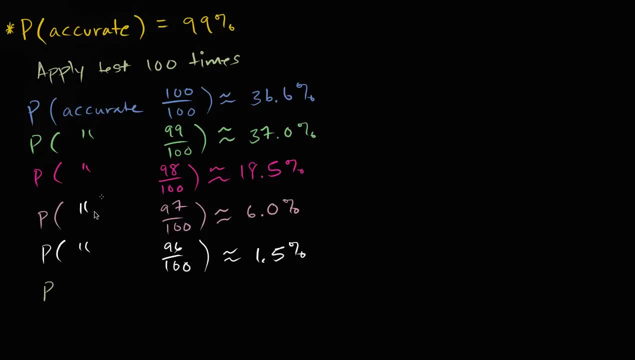 you just get super unlucky and that you know very few of them are accurate. But I'll just- and you see, you see what's happening to the probabilities as we have, as we have fewer and fewer of them being accurate, It becomes less and less probable. 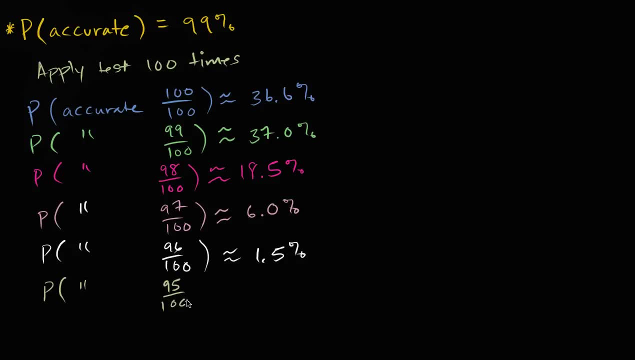 So the probability that 95 out of the 100 are accurate is is 0,, approximately 0.3%. So this was just kind of a- I guess you could say- a thought experiment If we had a test that we know for sure. 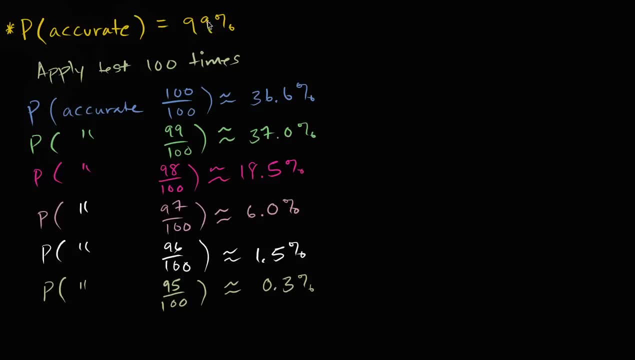 that every time you administer it, the probability that it's accurate is 99%, then these are the probabilities: that if you administer it 100 times that you get 100 out of 100 accurate. The probability that you get 99 out of 100 accurate. 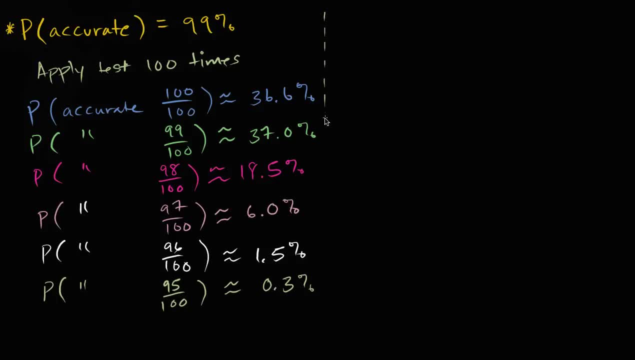 and so on and so forth. So let's just keep that in mind and then think a little bit about hypothesis testing and how we can use this framework. So let's put all that in the back of our minds And let's say that you have. 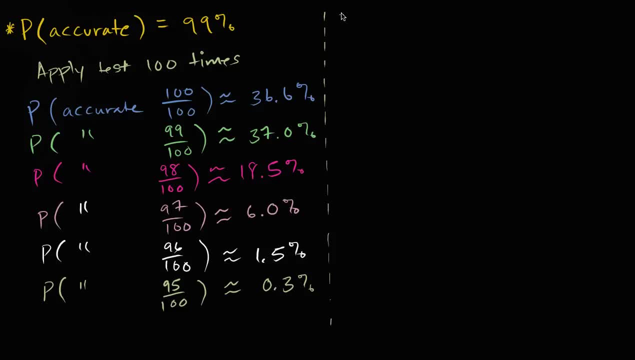 you have devised a new test. You have a new test and you don't know how accurate it is. You have a new cholesterol test. You don't know how accurate it is. You know that in order for it to be approved by whatever governing body, 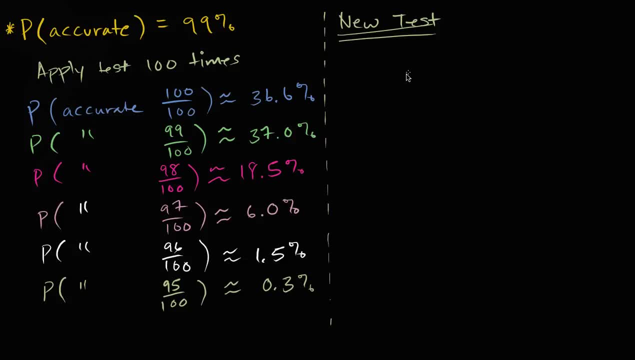 it has to be accurate 99,. the probability of it being accurate has to be 99%. So needs needs to have have probability of accurate accurate equal to 99%. You don't know if this is true, You just know that that's what it needs to be. 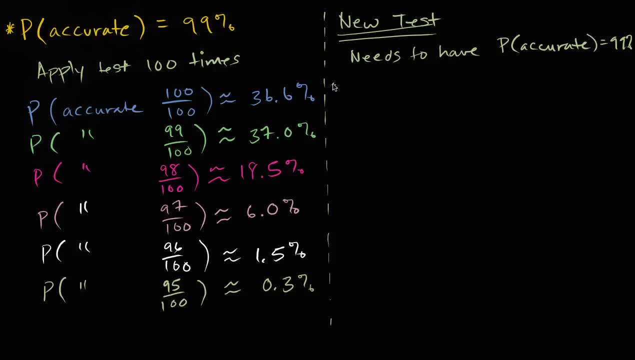 And so you have your test and let's say you set up a hypothesis and your hypothesis could be a lot of things, and once you get deeper into statistics, there's null hypothesis and alternate hypotheses. But let's just start with just a simple hypothesis. 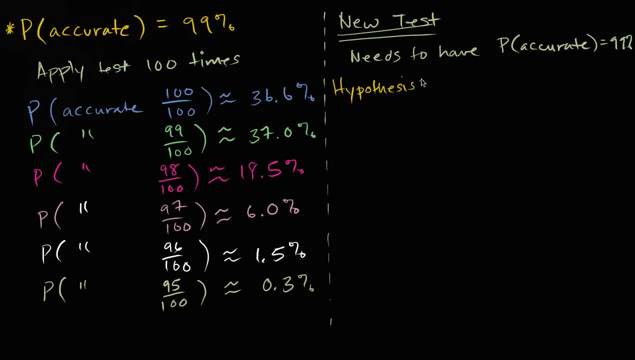 You're, you're hopeful. Your hypothesis is that that the probability that your new test, new test, is accurate, is accurate is. this is your hypothesis, Because you, you want that to be your hypothesis, because if you, if you feel good about it, 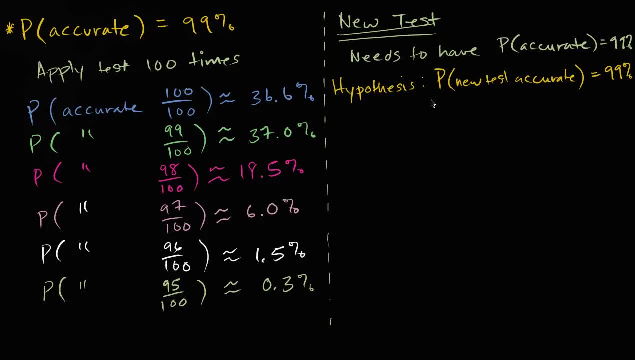 then you're like, okay, yeah, maybe I'll get approved by the appropriate governing body. So you say, hey, I, I. my hypothesis is that my new test is accurate 99, the probability of it being accurate is 99%. 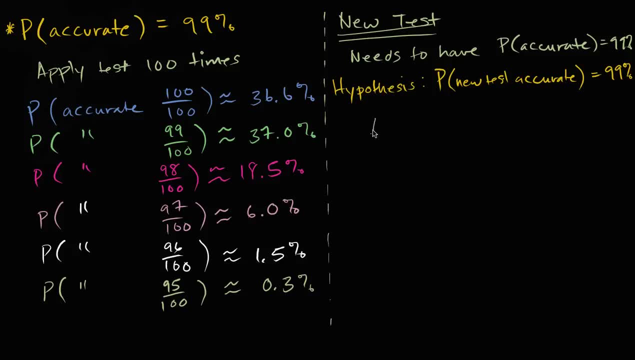 So then you go off and you apply it 100 times. So you apply your new test. You don't know the actual probability of it being accurate. You, you apply the test. You apply the test 100 times And let's say, out of those 100 times, 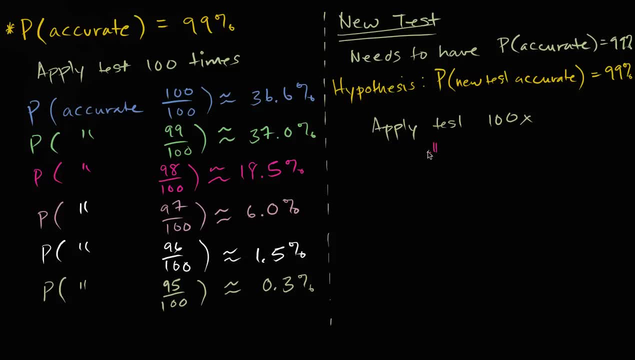 you get that they are accurate. You get that it is accurate and you're able to use some other test that you you know, some for sure test, some super accurate test, to verify your own test results And you see that it's an accurate 95 out of the 100 times.